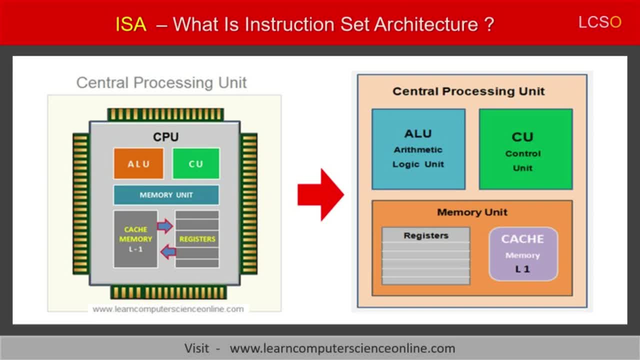 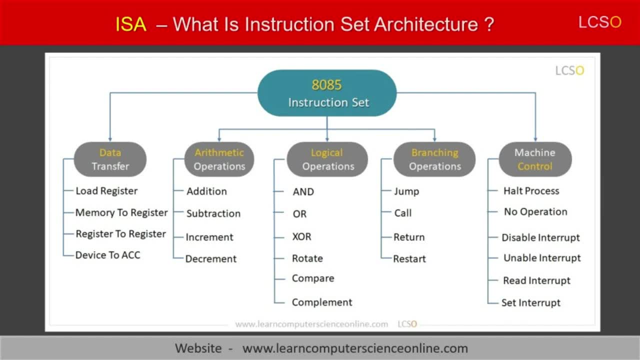 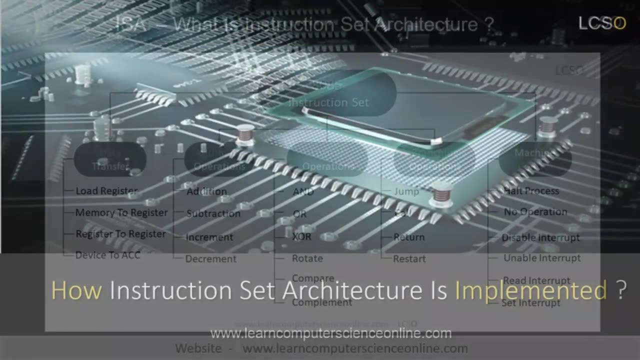 the operational capacity of the processor in terms of set of commands that the processor can decode and execute. For example, the Intel 8085 instruction set architecture consist of total 246 operation codes and 74 instructions. Let us now talk about how instruction set architecture is implemented into the processor. 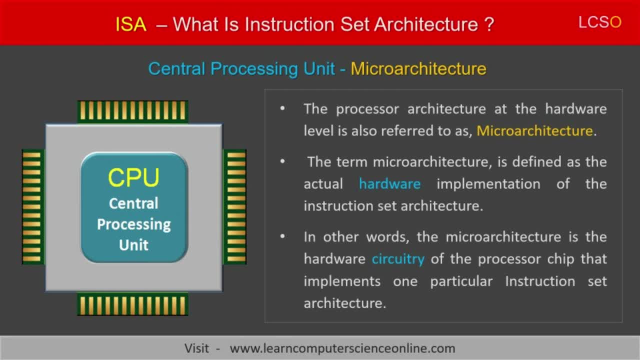 design. The processor architecture at the hardware level is also referred to as micro-architecture. The term micro-architecture is defined as the actual hardware implementation of the instruction set architecture. In other words, the micro-architecture is the hardware circuitry of 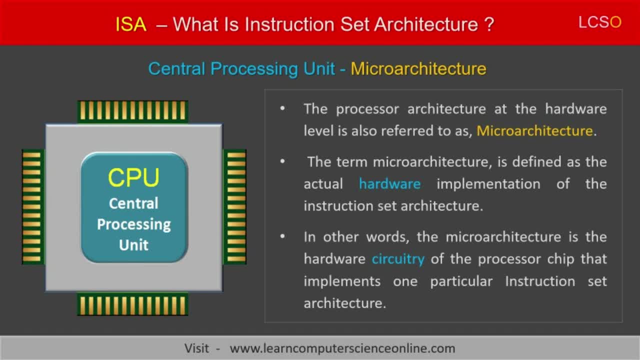 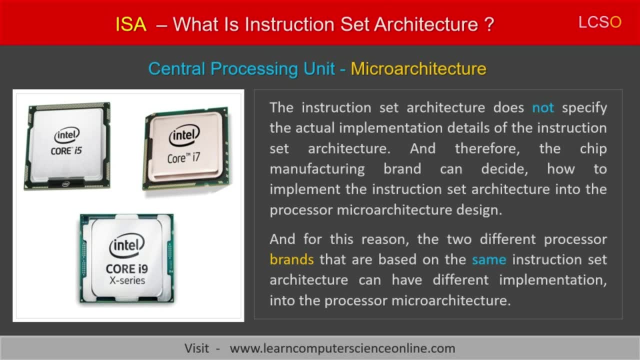 the processor chip that implements one particular instruction set architecture. The instruction set architecture does not specify the actual implementation details of the instruction set architecture. Therefore, the chip manufacturing brand can decide how to implement the instruction set architecture into the processor micro-architecture design. 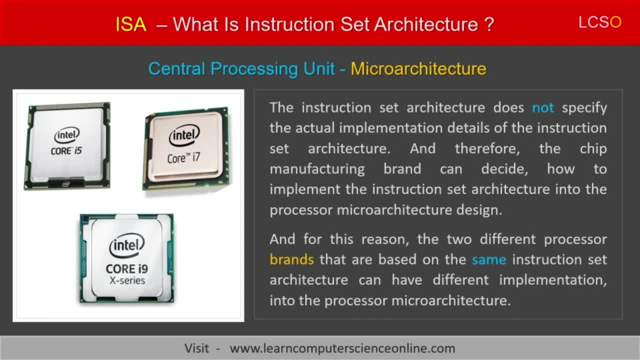 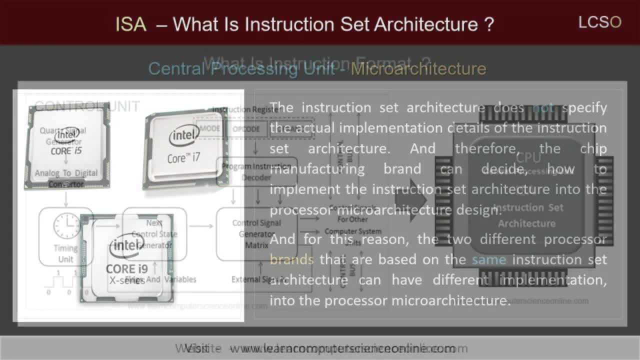 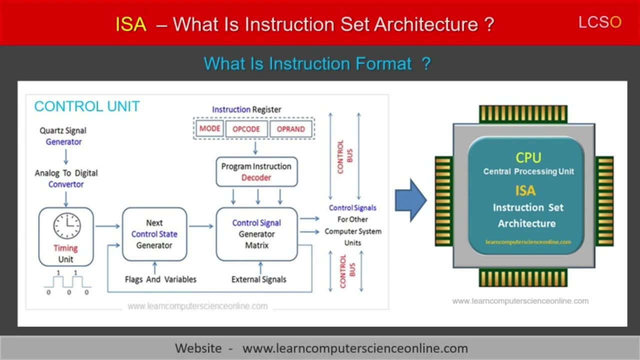 For this reason, the two different processor brands that are based on the same instruction set architecture can have different implementation into the processor micro-architecture. Alright, So far we have defined and understood the concept of the instruction set architecture and how it is implemented into. 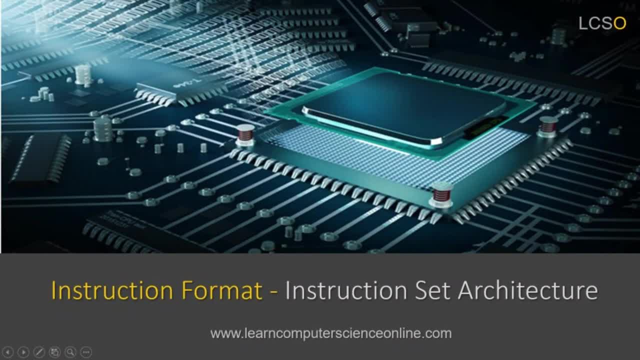 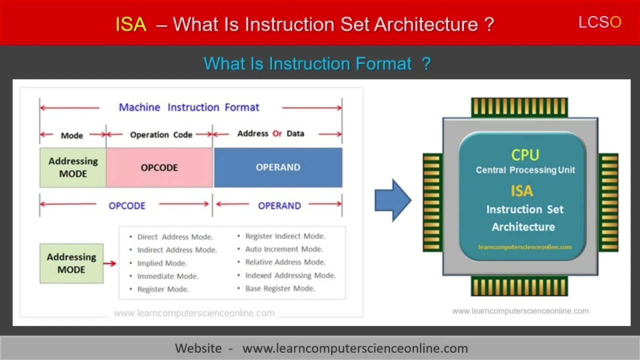 the processor micro-architecture. Let us now briefly discuss some other important fundamental concepts related to the processor architecture and its correlation with the instruction set architecture. The instruction format is another important design concept that is part of the processor architecture. The computer program consists of set of instructions which directs 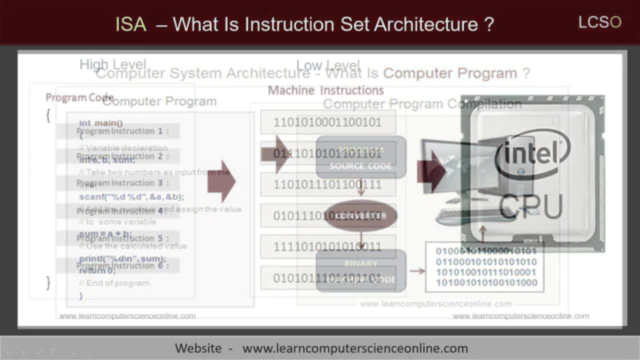 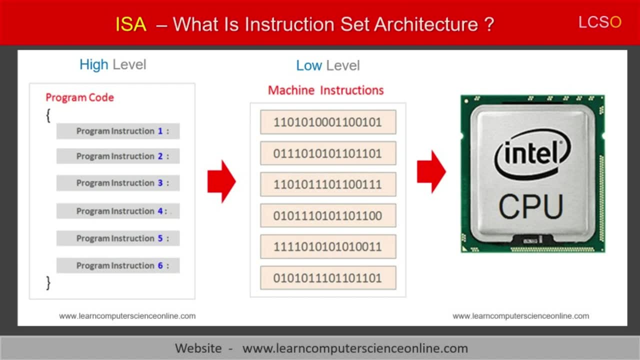 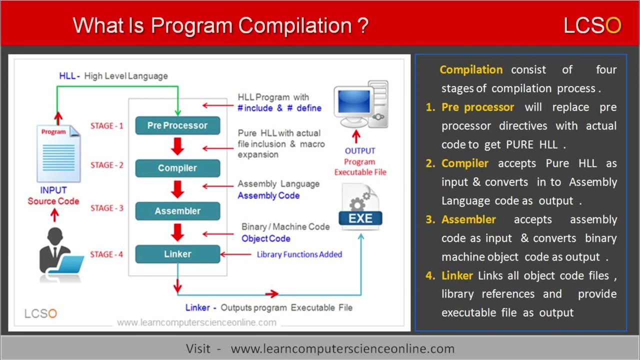 the CPU to perform some specific operations. However, we all understand that the computer can execute only low-level machine instructions in the binary format, And therefore all high-level programs are first compiled with the help of a special software called the compiler. 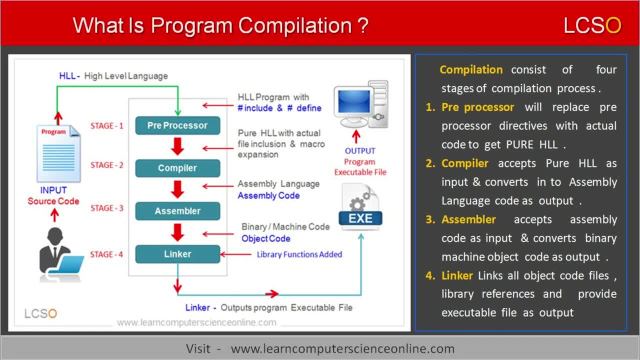 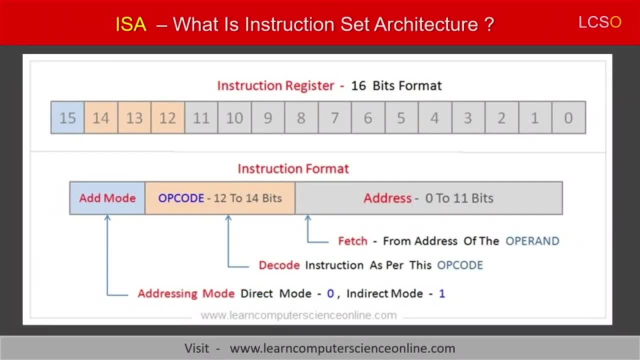 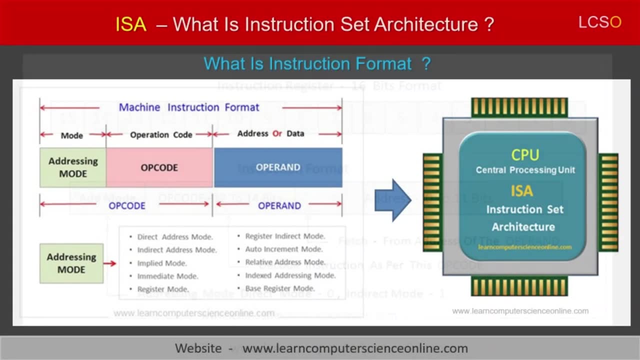 The compiler translates the high-level program instructions into the low-level machine instructions in the binary format. The instruction format basically defines the layout of the computer. The instruction format basically defines the layout of the machine instruction in terms of operation code, operand and the addressing mode. The